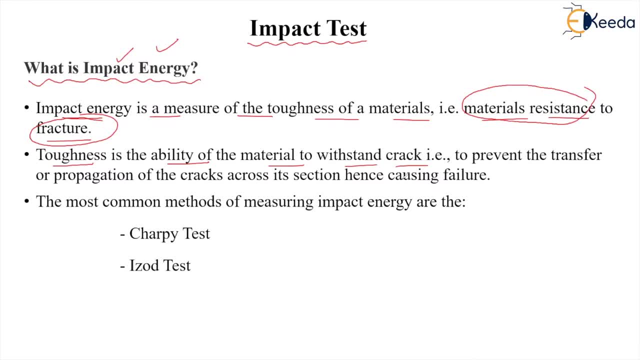 right. so whenever a failure takes place, first a crack initiates and that crack propagates and the final failure takes place. so what is the ability of the material to withstand that crack, to hold that crack for the longer time? that is called the toughness of the material. so toughness is the 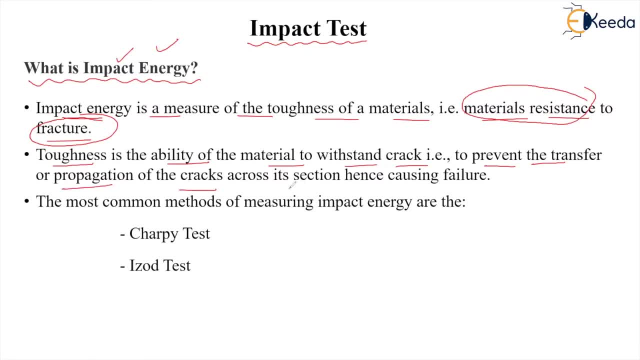 prevention of the propagation of the crack across the section before the failure takes place, right? so impact energy is basically the energy associated with the fracture or failure of the material right. what is the energy required to fill the material right? so we will discuss this thing in this chapter. so 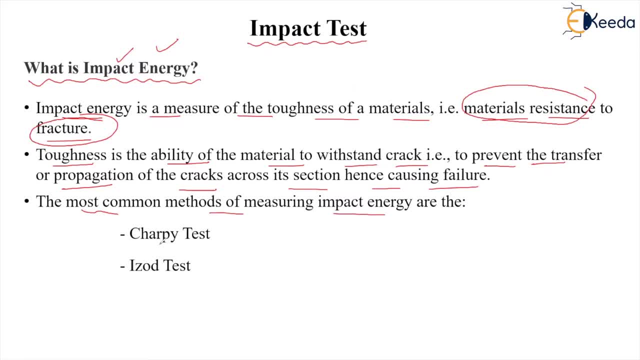 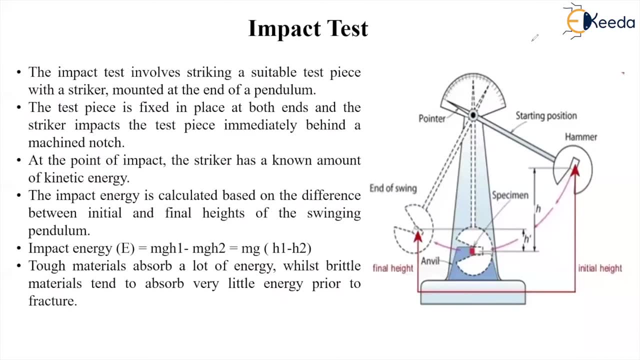 mainly, there are two types of tests for impact testing. this is charpy test and iso test. so we will discuss in coming lectures about this. let us now discuss how the impact test is done. in impact test we have a testing setup in which there is a specimen you can see here. 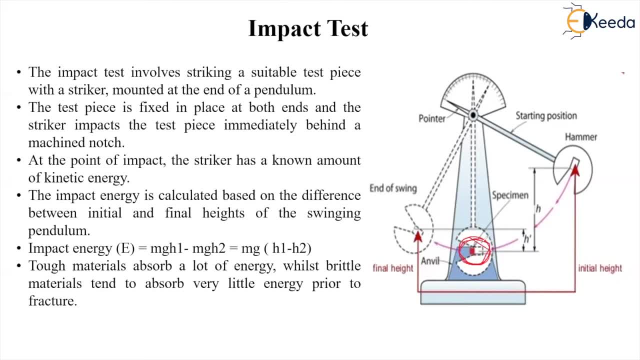 there is a specimen, the specimen we want to break. there is a hammer. there is a heavyweight hammer which strikes the this specimen and breaks the specimen. so initially it is having some potential energy, initially it has some datum- the height above the reference line- so initially it is having some datum- suppose h1 is the height- and initially it has some energy. that is called 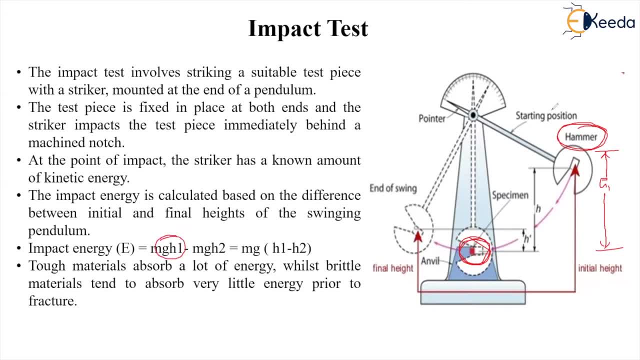 mgh1 potential energy. when the hammer is released from the starting position, it gains some kinetic energy, some kinetic energy again. that kinetic energy breaks, imparts a impact on the specimen and this specimen breaks and some of the there is some swing in on other another side of the, this machine. 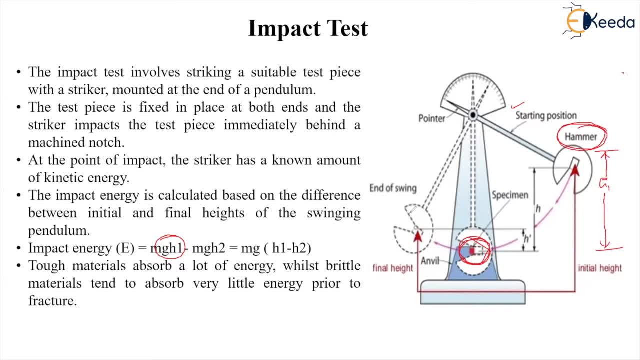 another part of this machine and there is the. the height up to which it raises, decreases. you can see here: initially it was h, finally it was h- or h1 and h2, right suppose final energy is mgh2. so there is decrease in potential energy of the initial and final energies. that is mgh1 minus. 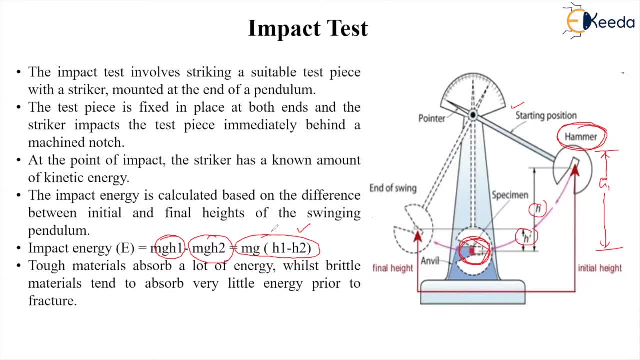 mgh2 right. this energy is the basically the lowest. the difference in this energy is basically impact energy, which is which is used to crack or break the specimen and this is the toughness of the material or energy used to break the material right. so this is called the impact energy. 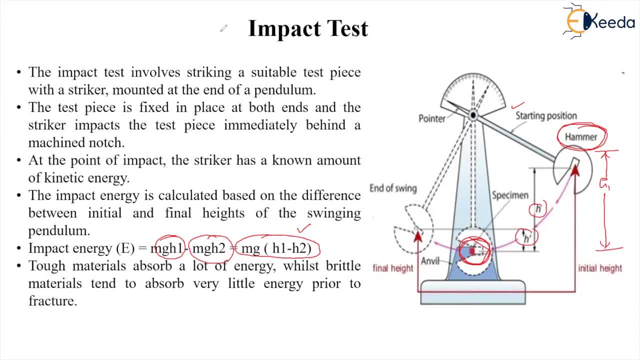 so impact test. so here, impact test involves striking a suitable test piece with a striker. striker is basically hammer, striker is basically hammer mounted at the end of the pendulum. this is like a pendulum right: that test piece is fixed in a place at both ends and striker impacts the 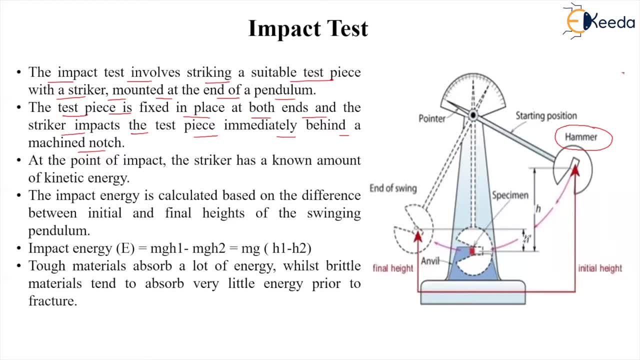 test piece immediately behind a machine notch. so this is a notch, this is and this is a type of notch, right, you can see here, v-shape, v-shape. something is seen which is a notch, notch of this striker as well as notch of the specimen also. we can also make 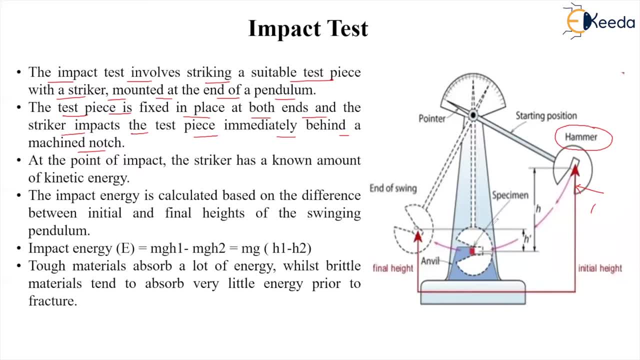 the note of the specimen, also right. so here you can see it is not visible. there is a notch of the specimen, also right. so behind the machine notch, at the point of the impact, the specimen striker has a known amount of kinetic energy. and where this kinetic energy is known? because this 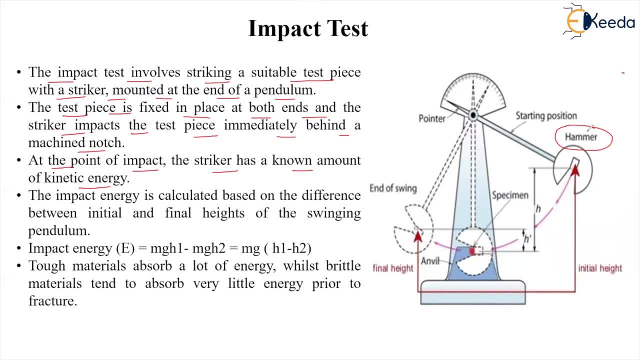 kinetic energy is obtained from the decrease in potential energy. whatever there is decrease in potential energy, that equals the kinetic energy, right. so the impact energy is calculated based on the difference between the initial and final heights- right two potential energies of the swinging envelope, right. so this is the basically the impact energy. tough materials absorb a lot. 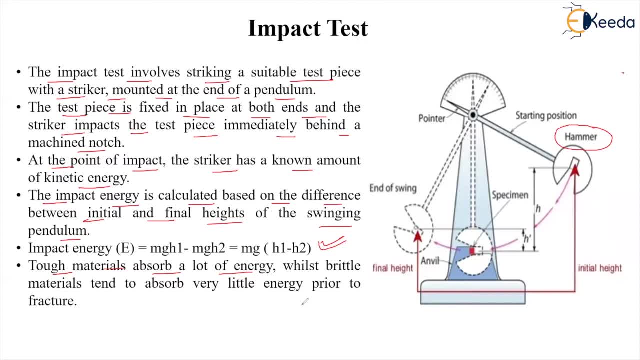 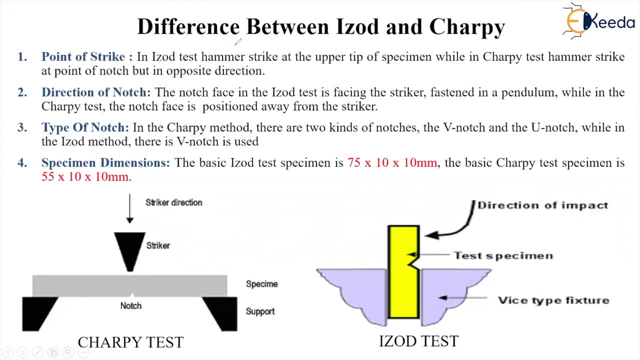 of energy. if the material is tough, it will absorb a lot of energy, right, and if the material is brittle- material like- tend to absorb very little energy prior to fracture. so this is how we obtain the impact energy and this is the impact estimation. so here there is a difference. 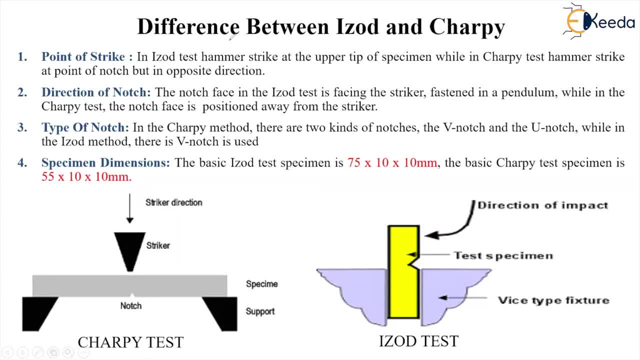 between? we have already discussed. there are two types of tests. are there impact test, that is, the impact testing machine, and the impact testing machine and the impact testing machine is Izod test and Charpy test, right? so what is difference between two tests? one is a point. 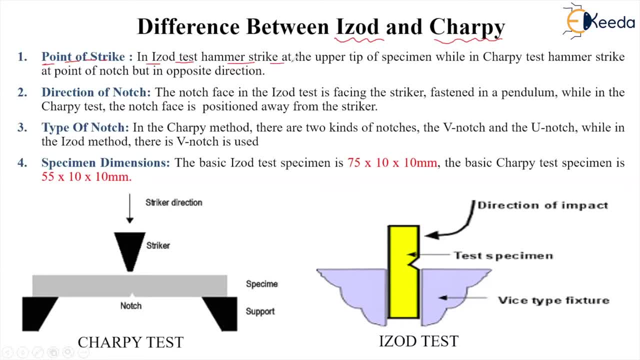 of strike in Izod test hammer strikes the upper tip of the specimen in Izod test. you can see here. this is the upper tip, which is at which the hammer strikes, while in Charpy test hammer strikes at a point of notch, but in opposite direction. here you can see here. 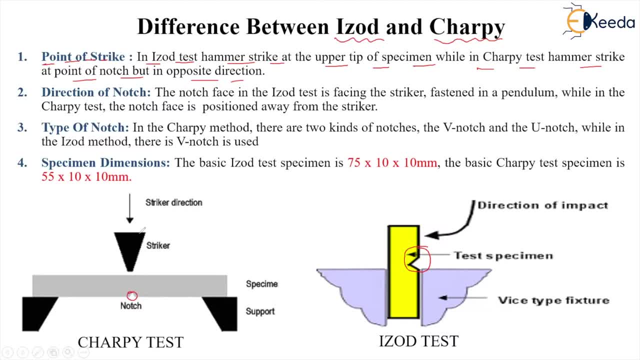 this is the notch, this is the notch and striker strikes at the point of notch but opposite direction. the direction is opposite, it is not at the notch, it is at the opposite of the notch right. so second difference is direction of notch. the notch face in Izod test facing. 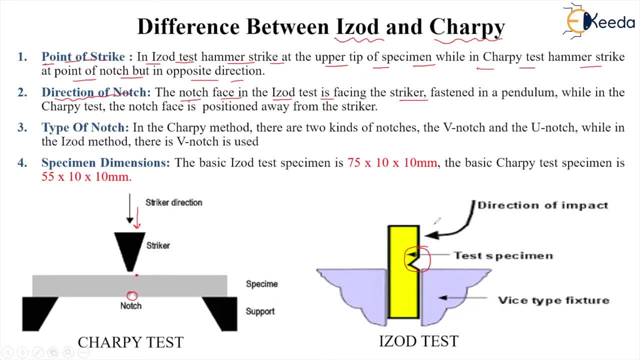 the striker. you can see here, the striker is there and notch is here. both are facing each other, while in Charpy test the notch face is positioned away from the striker. here. you can see here two faces are opposite: striker and notch are at different faces. so direction. 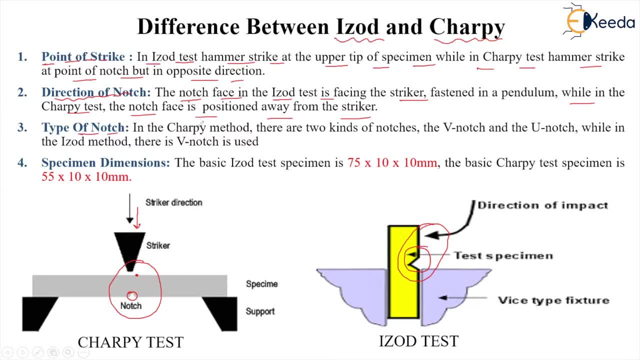 is different type of notch. another point of difference that Charpy test are of two kinds of notches. are there V notch and U notch? in Charpy test we can use V notch and U notch, while in Izod test we use generally V notch. so here we use the V notch, right? 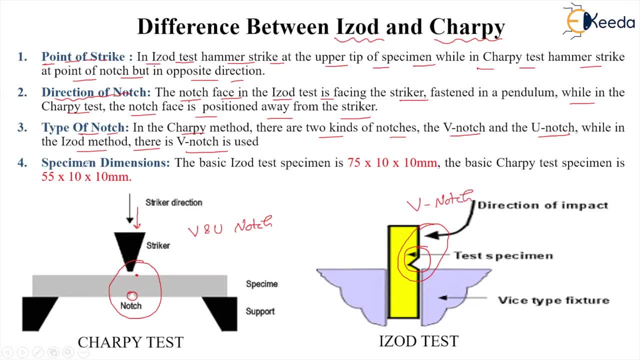 and in Charpy test we can use V and U notch. another is the specimen dimensions. some fixed dimensions are there, although it is not always fixed, but some standard dimensions are there. for Izod test the dimensions are this: 75 by 10 by 10 millimeter of specimen is there and 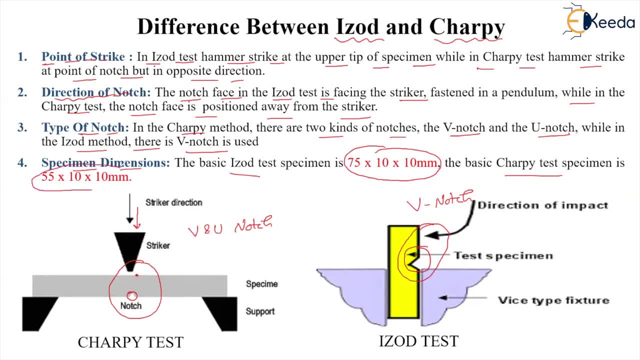 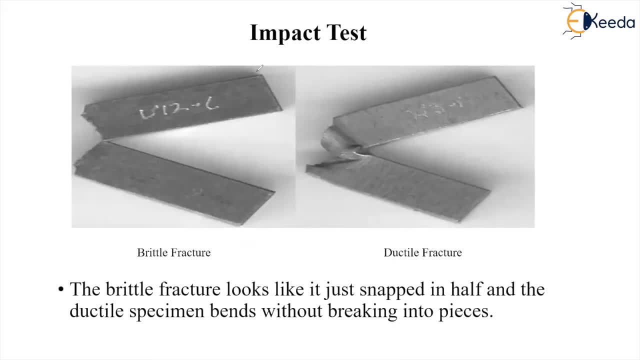 for Charpy test the specimen dimensions are 55 by 10 by 10 millimeter. so this is the difference between Charpy and Izod test. there is a practical demonstration after the breaking of the part. there are two types of fractures are shown here. that impact test is done on two materials. one is a brittle fracture. 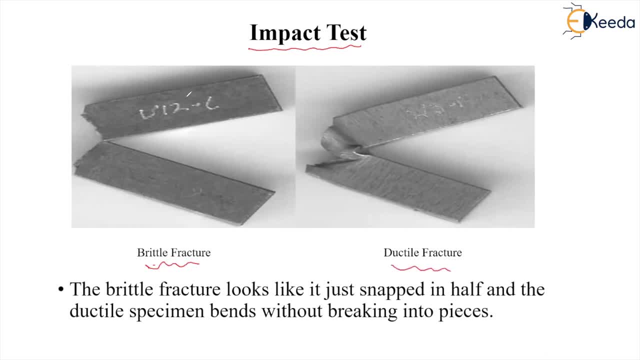 and another is a ductile fracture. you can see here in brittle fracture the two parts of the specimen is divided into two parts separately. it is seen in separate parts like this right and in ductile fracture. this is the specimen only bends. it do not break. clearly right. it bends right and the molecules are.